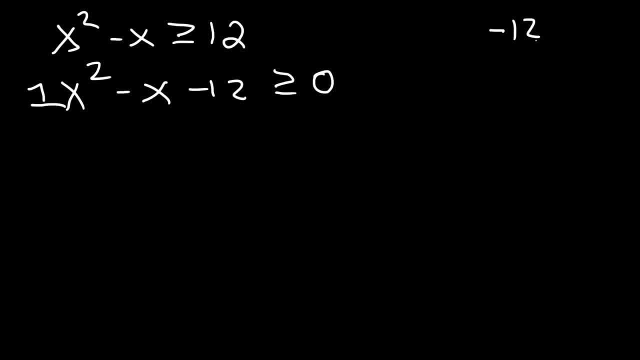 We need to find two numbers that multiply to the constant term negative 12, but add to this The middle coefficient is negative 1. And those two numbers will be negative 4 and 3.. Negative 4 times 3 is negative 12, but negative 4 plus 3 is negative 1.. So to 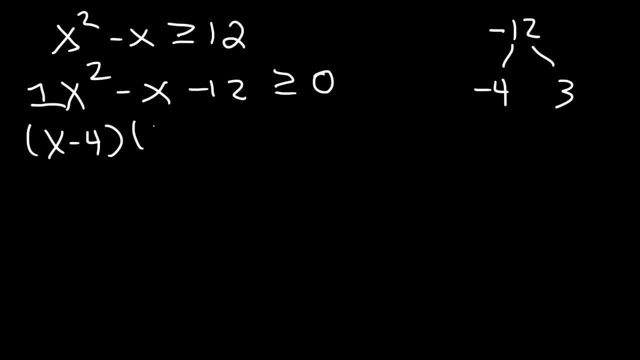 factor it, it's going to be x minus 4 times x plus 3.. Now if we set each factor equal to 0, there's two points of interest that we need. If we add 4 to both sides, we can see that x is. 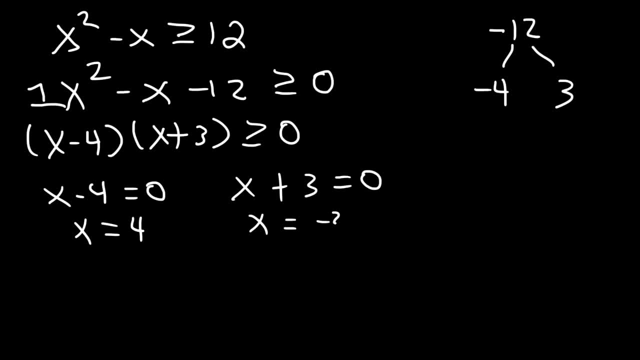 4, and if we subtract 3 from both sides, x is negative 3.. So let me write that x can be 4 and negative 3.. And the reason why it can equal those numbers is because here it's greater than or equal to 0.. Now we need a number line in order. 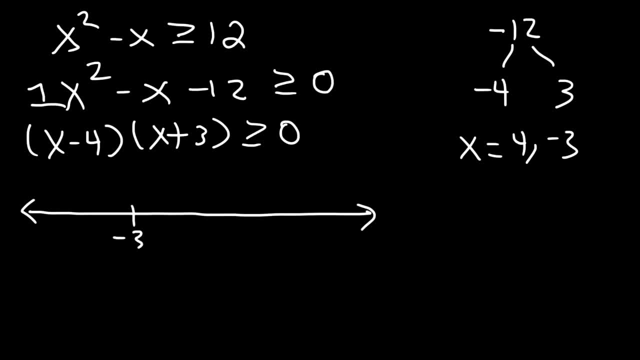 to get the right answer. So we have negative 3 on the left and 4 on the right. At the end, on the right side, we have 4 on the left and 4 on the right side. we have positive infinity and negative infinity on the left. Now, since the solution, 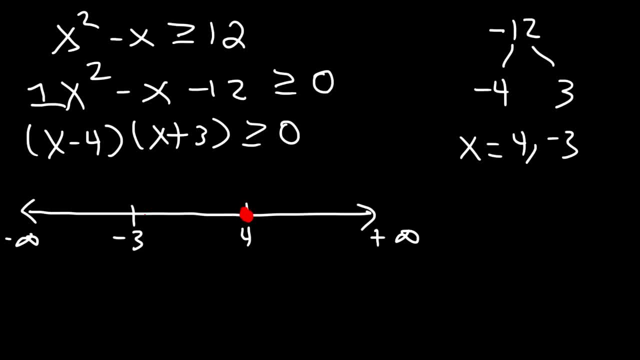 includes 4 and negative 3, I'm going to put a closed circle at those points. If it doesn't include those points, you need to write an open circle. Now the solution: well, the product of these two factors has to be greater than 0 or equal to it. So we need to check these three. 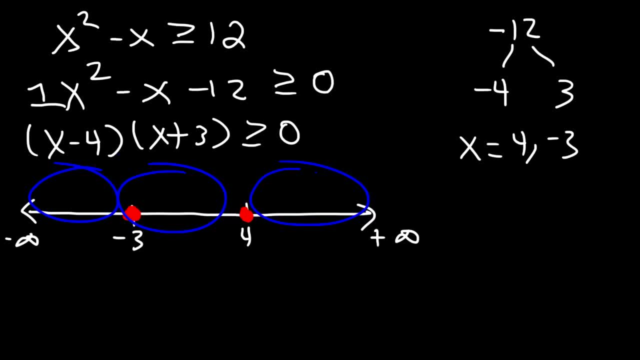 regions to see when this side of the equation is positive. We don't want the part where it's negative because it has to be greater than 0. So we got to plug in numbers and test the signs. So let's pick a number between 4 and infinity. Let's try 5.. So if we plug in 5 into this, 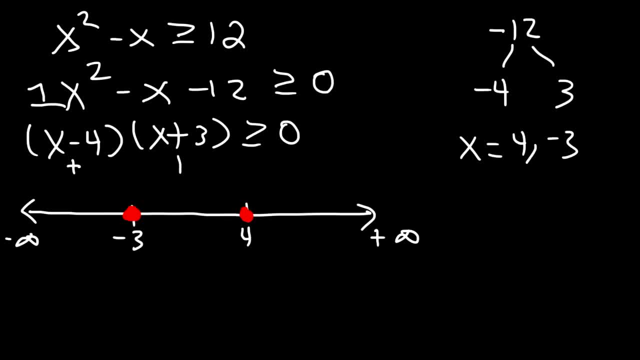 expression: 5 minus 4 is positive. 5 plus 3 is positive. When you multiply two positive numbers, it will give you a positive result. Now let's pick a number between negative 3 and 4.. 0 is a good number. 0 minus 4. 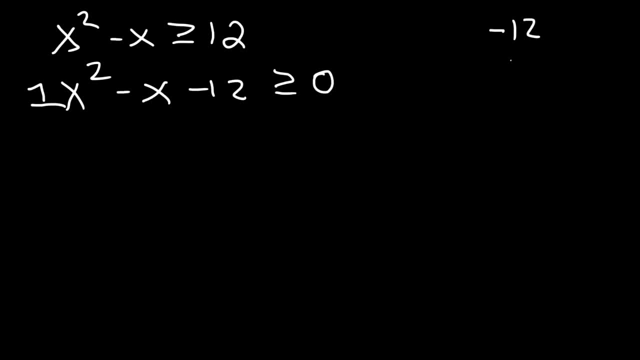 We need to find two numbers that multiply to the constant term negative 12, but add to this trinomial. We need to find two numbers that multiply to the constant term negative 12, but add to this middle coefficient negative 1. And those numbers will be negative 4 and 3.. 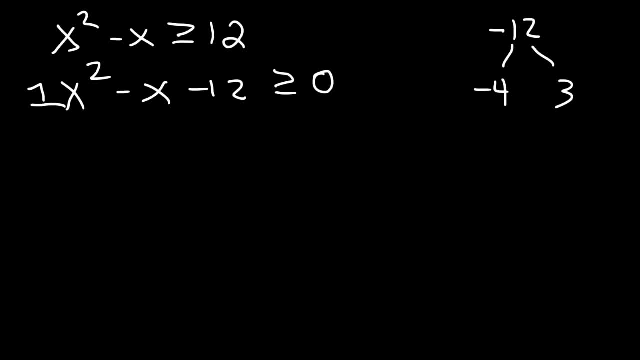 Negative 4 times 3 is negative 12.. And negative 4 plus 3 is negative 1.. So to factor it, it's going to be x minus 4 times x plus 3.. Now if we set each factor equal to zero, there's two points. 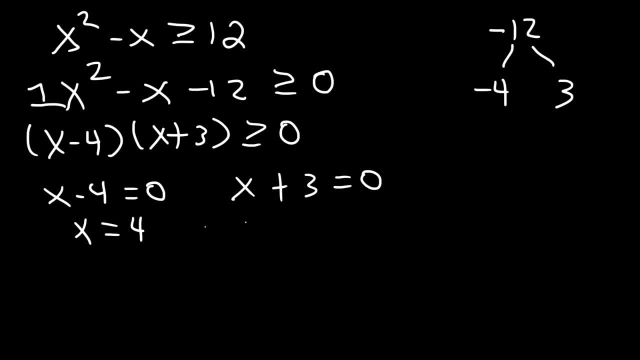 of interest that we need. If we add 4 to both sides, we see that x is is 4, and if we subtract 3 from both sides, X is negative 3. so let me write that X can be 4 and negative 3, and the reason why it can equal those numbers is: 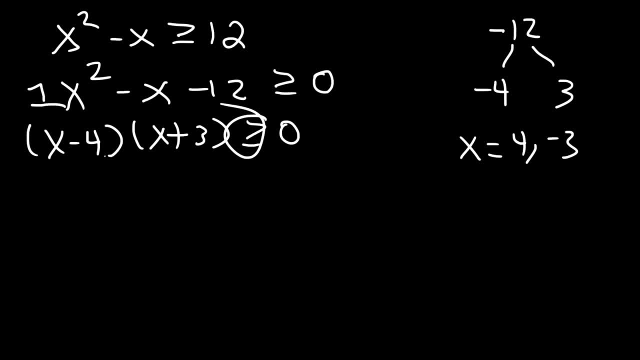 because here it's greater than or equal to 0. now we need the number line in order to get the right answer. so we have negative 3 on the left and 4 on the right. at the end, on the right side, we have positive infinity and negative. 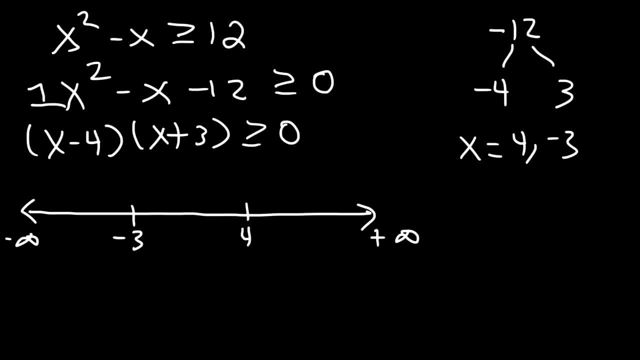 finity on the left. now, since the solution includes 4 and negative 3, I'm going to put a closed circle at those points. if it doesn't include those points, you need to write an open circle. now the solution: well, the product of these two factors has to be greater than 0 or equal to it. so we need to check. 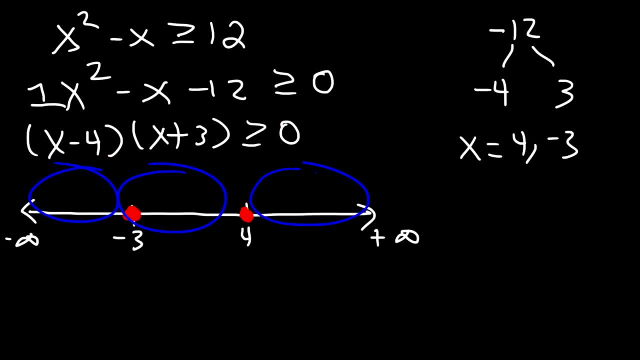 whether the number line is greater than 0 or equal to 0. so we need to check whether the number line is greater than 0 or equal to 0. so we need to check these three regions to see when this side of the equation is positive. we 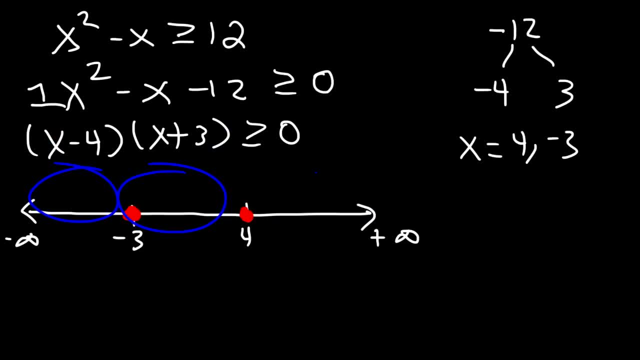 don't want the part where it's negative because it has to be greater than 0. so we got to plug in numbers and test the signs. so let's pick a number between 4 and infinity. let's try 5. so if we plug in 5 into this expression, 5 minus 4 is 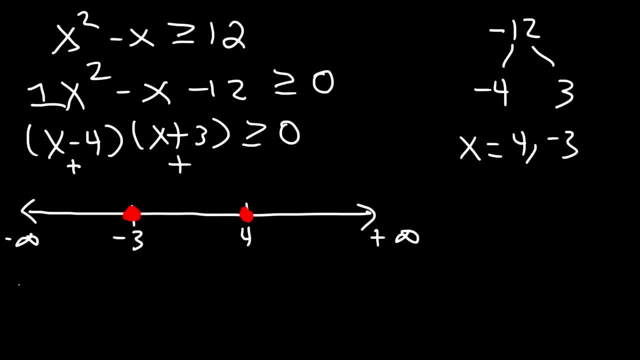 positive. 5 plus 3 is positive. when you multiply 2 positive numbers, it will give you a positive result. now let's pick a number between negative. 3 and 4. 0 is a good number. 0 minus 4 is negative. 0 plus 3 is positive. a negative number times a. 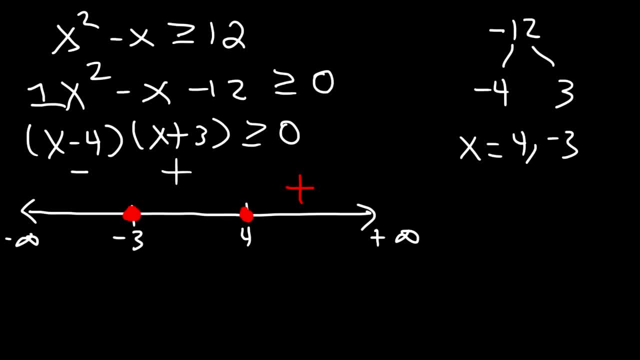 is negative. 0 plus 3 is positive. A negative number times a positive number will give you a negative result. So let's put a negative sign Now. let's try a number between negative infinity and negative 3, like negative 4.. Negative: 4 minus 4 is negative. Negative 4 plus 3 is negative. 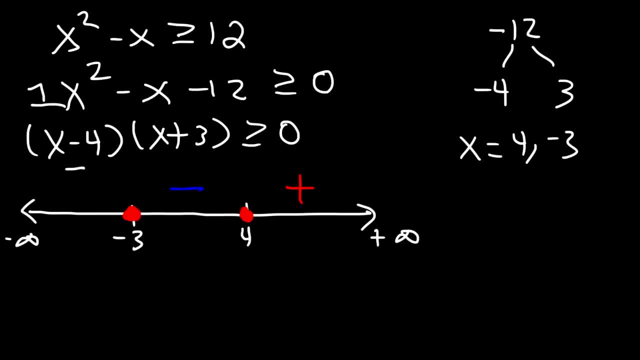 And so if you multiply two negative numbers, you get a positive result. So let's put a negative sign. If you multiply two negative numbers, it will give you a positive number. Now notice that the multiplicity of the first 0,- 4 is 1, and the multiplicity for the 0, negative 3 is also 1.. Whenever the exponent 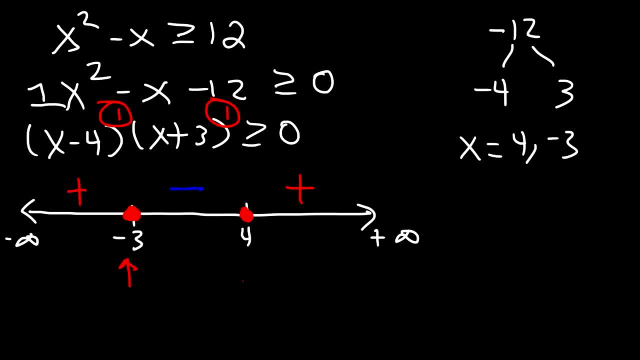 or the multiplicity is odd. the sign will change at that point. So if you know the first sign, you can easily determine the rest. So for this 0,. the multiplicity is odd, So it's going to switch from positive to negative. 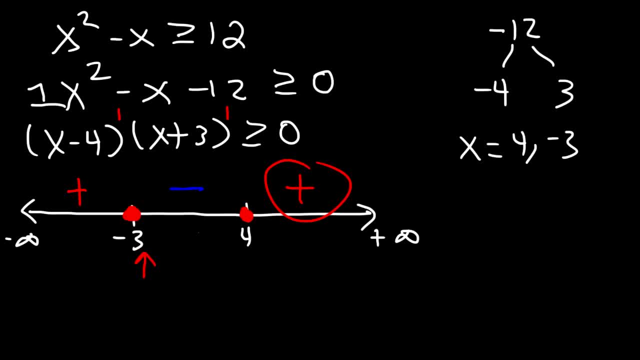 And for this 0,. the multiplicity is also odd, So it's going to switch from negative to positive. But if it was even, it won't change sign. So that's something to keep in mind. Now we're looking for the region where it's positive, So we need to shade this region. 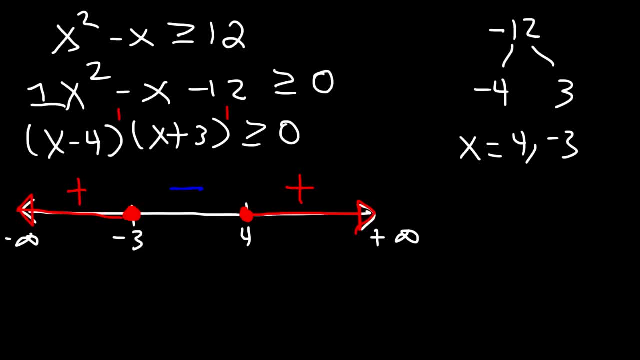 and the region on the left. So to write the answer using interval notation, it's going to be a negative infinity. It's a negative 3.. Now it includes a negative 3. So we need to use a bracket instead of. 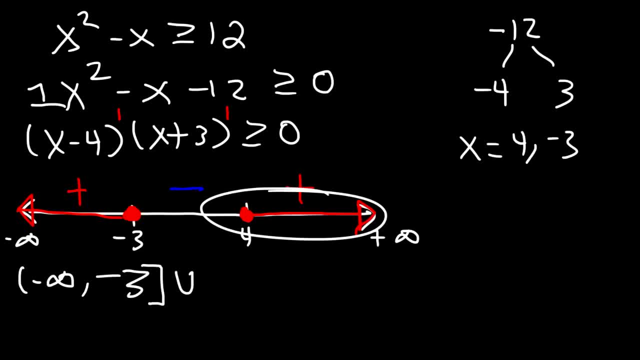 a parentheses And then union for the second part. It's going to start back up at 4 and go to infinity. So as an inequality, you can write the answer this way: You can say S, I mean the S, but X is less than or equal to negative 3.. And then you can write or: 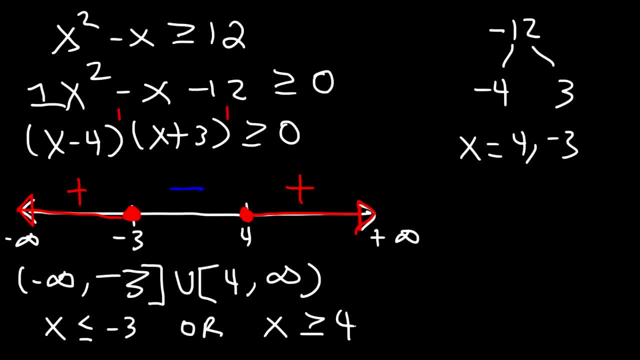 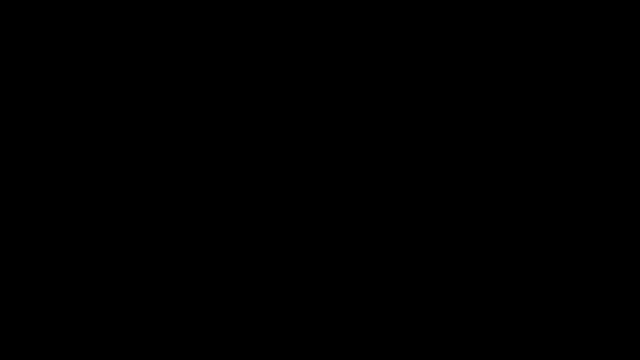 X is equal to or greater than 4.. So you can represent it using interval notation or using inequalities, And that's it. So that's how you can solve a quadratic inequality. Let's try another example. So let's say, if we have X squared plus 9.. 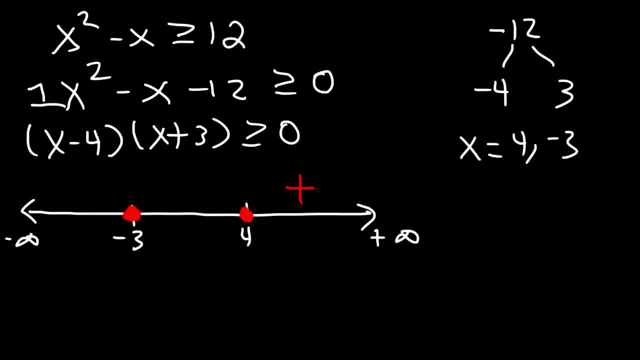 positive number will give you a negative result. so let's put a negative sign now. let's try a number between negative, infinity and negative. 3 like negative, 4 negative, 4 minus 4 is negative, negative 4 plus 3 is negative. and so if you 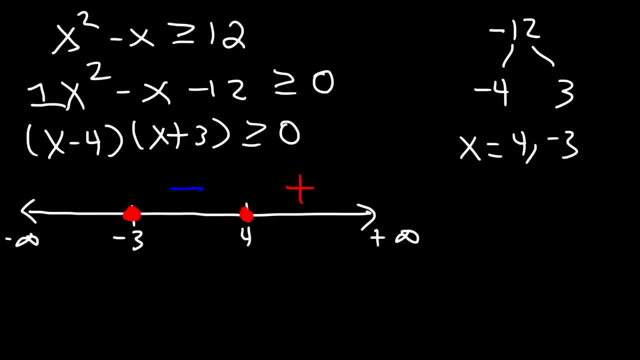 multiply two negative numbers, it will give you a positive number. now notice that the multiplicity of the first 0- 4 is 1 and the multiplicity for the 0 negative 3 is also 1 whenever the exponent or the multiplicity is odd. the. 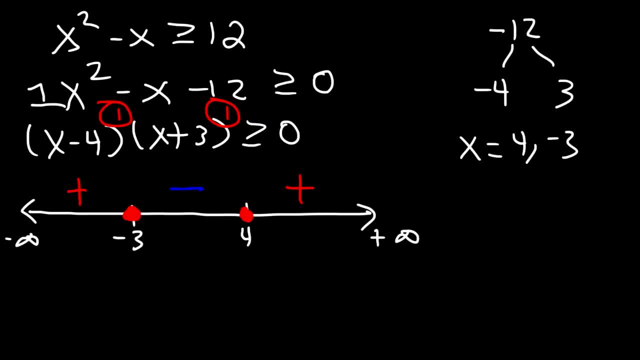 sign will change at that point. so if you know the first sign, you can easily determine the rest. so for this 0, the multiplicity is odd, so it's going to switch from positive to negative, and for this 0 the multiplicity is also odd, so it's going to switch from. 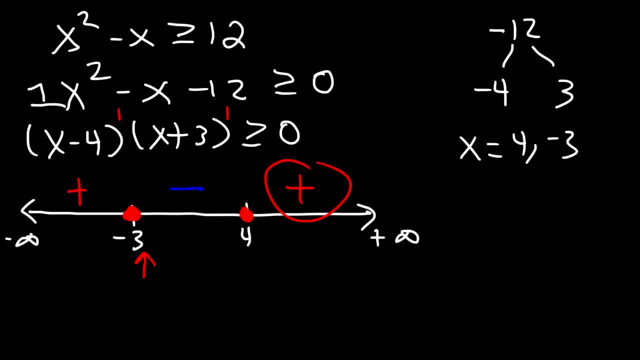 negative to positive, but if it was even, it won't change sign, so that's something to keep in mind. now we're looking for the region where it's positive, so we need to shade this region and region on the left. so to write the answer, use an. 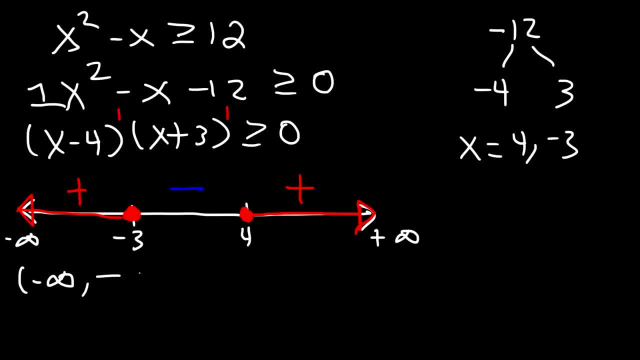 interval notation. it's going to be negative infinity to negative 3. now it includes negative 3, so we need to use a bracket instead of a parentheses and then union. for the second part it's going to start back up at 4 and go to infinity. so as an inequality, you can. 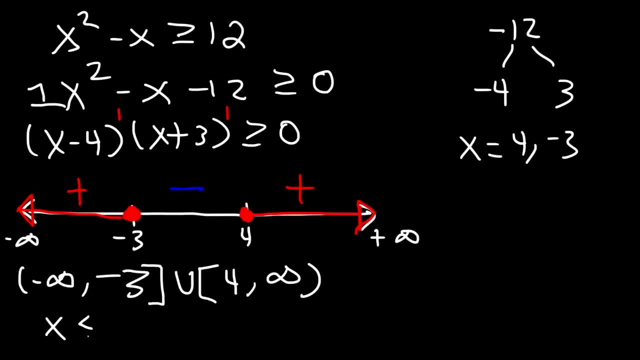 write the answer this way: you can say s- I mean the s- but X is less than or equal to negative 3, and then you can write: or X is equal to or greater than 4, so you have no variables that will set u. that's gonna be gotten a little bit more. 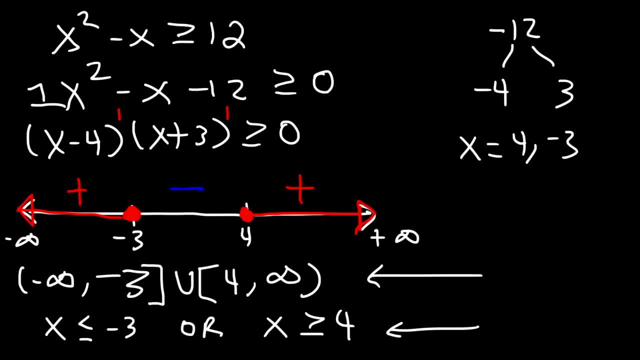 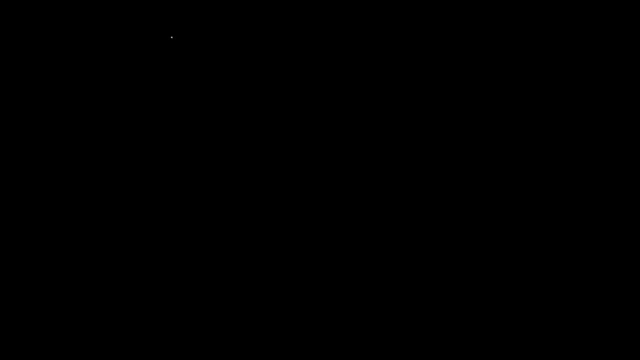 F used by the problem must be fixer. ok, so? so let's try to Solve a quadratic inequality. let's try another example. so let's say: if we have x squared plus nine, and we're gonna say that it's greater than six, X, go ahead and try this. 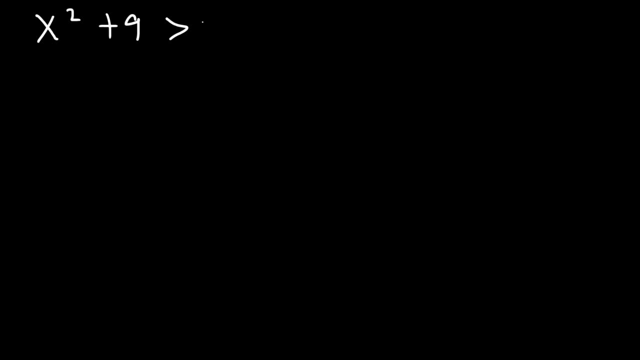 And we're going to say that it's greater than 6X. Go ahead and try this. So we need to get a 0. On one side of the inequality. So let's subtract both sides by 6X. So it's going to be negative 6X on the left side. Now we need to factor. 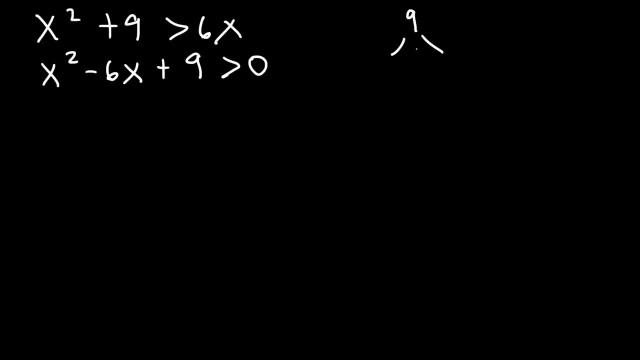 Two numbers that multiply to 9 but add to the middle coefficient negative. 6 is negative 3.. So it's going to be X minus 3 times X minus 3.. Now, because the two factors are the same, this trinomial is known as a perfect square trinomial, So we can write it as X minus 3. 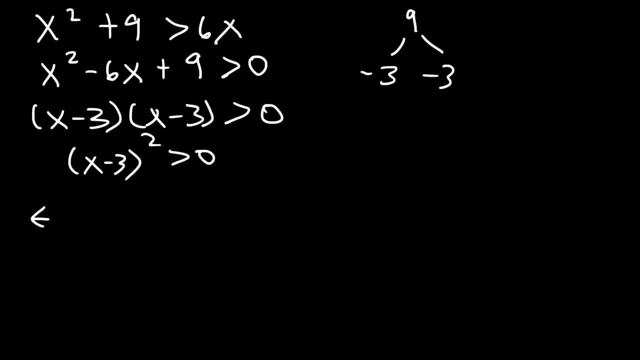 squared, Since we have two of them. So if you set X minus 3 equal to 0, you'll get X is equal to 3.. So we have one point of interest with two boundaries. Now notice that it's greater than 0 but doesn't equal to 0. So therefore, at 3, we have an. 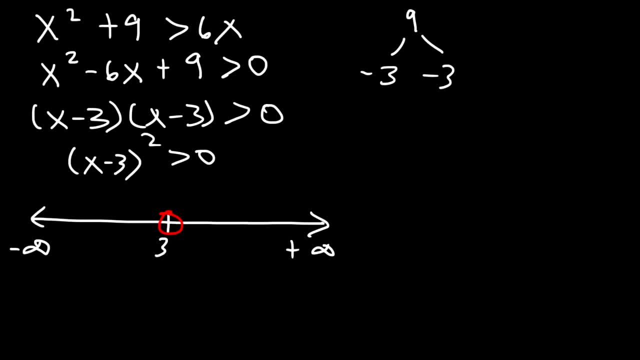 open circle, not a closed circle. So let's pick a number between 3 and infinity. If we plug in 4, 4 minus 3 is positive, And if you square a positive number, it will give you a positive result. 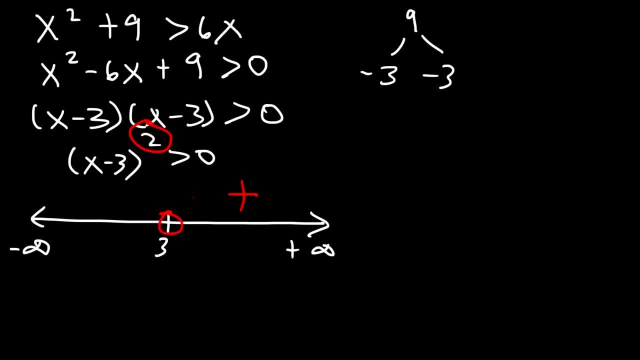 Now notice that the multiplicity is even. So as we go across this 0,, that is 3, the sign will not change, So then it's going to stay the same. On the left side it should be positive And to test it, 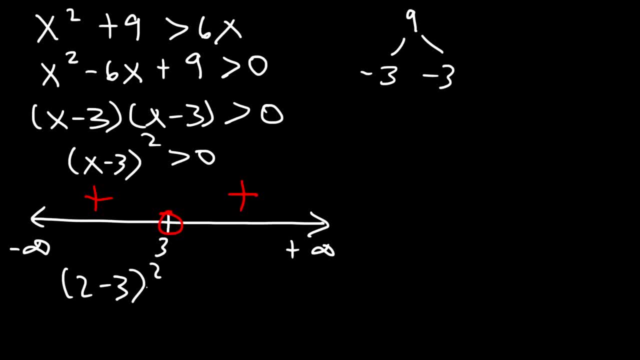 let's say, if you plug in 2. 2 minus 3 squared, 2 minus 3, is negative 1, but when you square a negative 1, you get a positive result. So it's always positive, except at 3.. At 3 is equal to 0.. 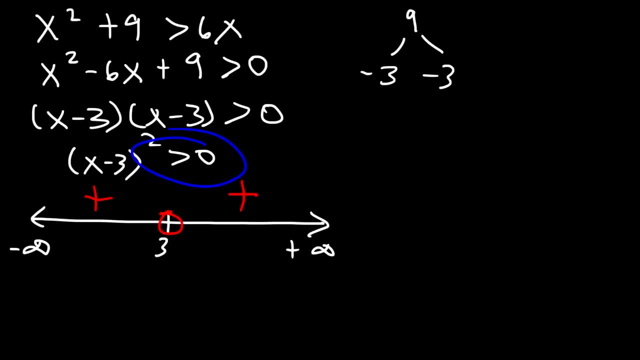 We only want the solutions where it's positive. So we need to shade the left side and also the right side, just not the middle. So therefore we can write the answer in interval notation as negative: infinity to 3, not including 3, union 3 to infinity, So as an. 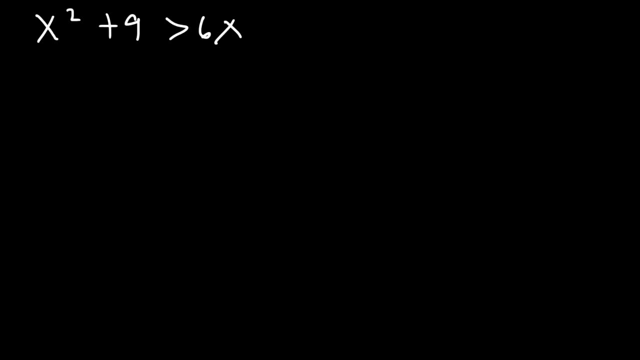 So we need to get a 0 on one side of the inequality. So let's subtract both sides by 6x, So it's going to be negative 6x on the left side. Now we need to factor Two numbers that multiply to 9 but add to the middle coefficient negative 6. 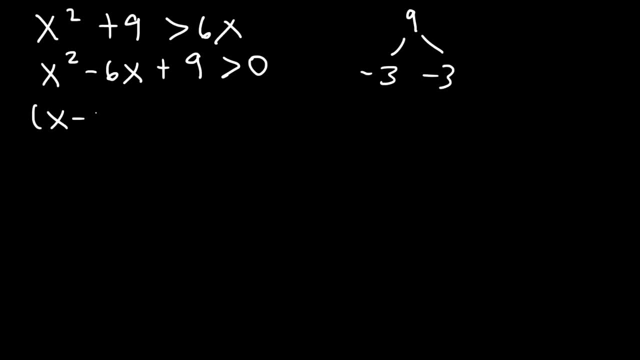 Is negative 3, So it's going to be x minus 3 times x minus 3. Now, because the two factors are the same, This trinomial is known as a perfect square trinomial, So we can write it as x minus 3 squared. 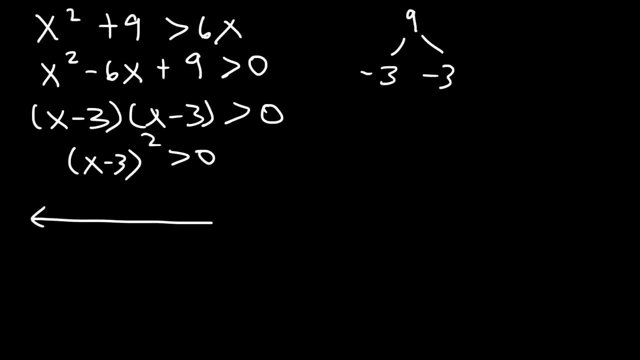 Since we have two of them. So if you set x minus 3 equal to 0, You'll get x is equal to 3. So we have one point of interest with two boundaries. Now notice that it's greater than 0 but doesn't equal to 0. 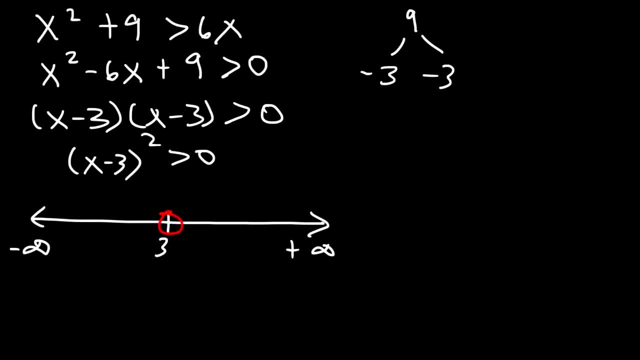 So therefore, at 3 we have an open circle, Not a closed circle. So let's pick a number between 3 and infinity. If we plug in 4, 4 minus 3 is positive, And if you square up A positive number, It will give you a positive result. 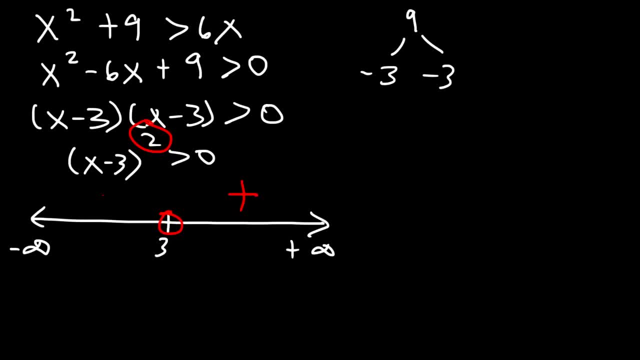 Now notice that the multiplicity is even. So, as we go across this arrow, That is 3, The sign will not change. So then it's going to stay the same. On the left side it should be positive. And to test it, Let's say, if you plug in 2. 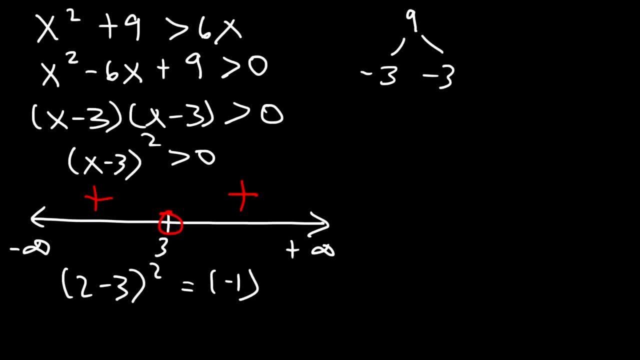 2 minus 3 squared 2 minus 3 is negative 1, But when you square negative 1 You get a positive result. So it's always positive, except at 3, That 3 is equal to 0. We only want the solutions where it's positive. 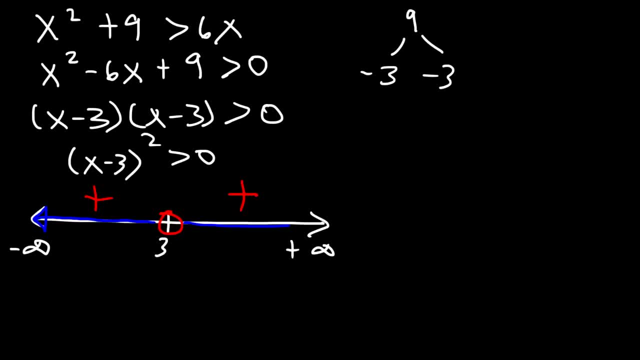 So we need to shade the left side And also the right side, Just not the middle. So therefore we can write the answer In interval notation as Negative infinity to 3, Not including 3, Union 3 to infinity. So as an inequality we can say that X is less than 3 or. 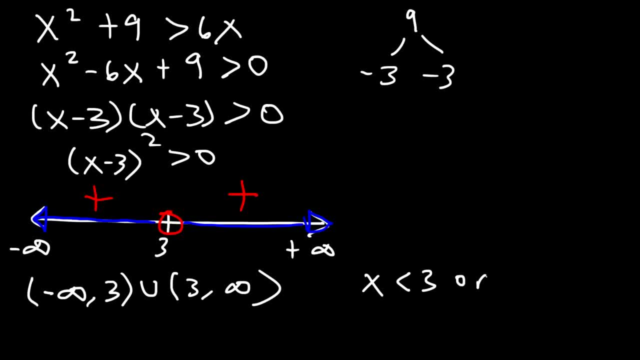 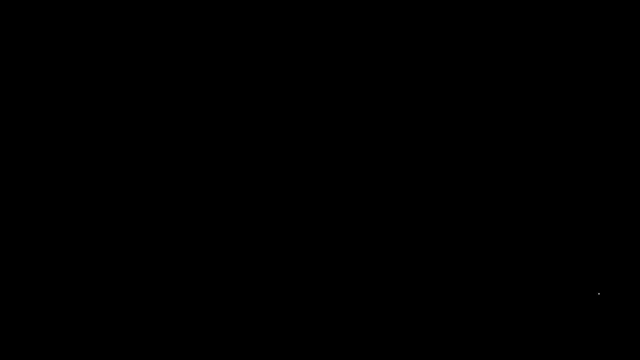 inequality. we could say that X is less than 3 or X is greater than 3, but it doesn't equal 3.. So that's the solution for this particular quadratic inequality. Now let's move on to our next example. So let's say that 2X squared is greater than X plus 6.. Go ahead and try that. 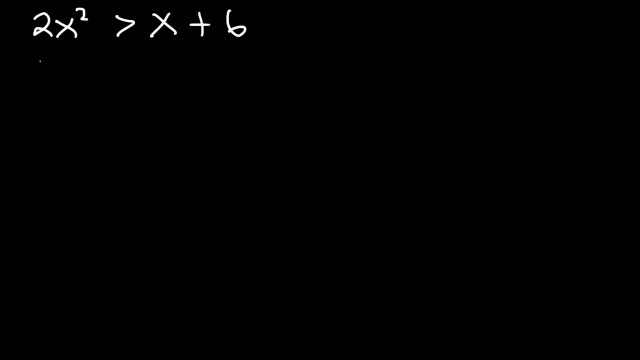 So let's move the X plus 6 from the right side to the left side, So on the left side they will be negative. Now we need to factor this expression. So how can we factor trinomial where the leading coefficient is not 1? First you need to multiply the leading coefficient and 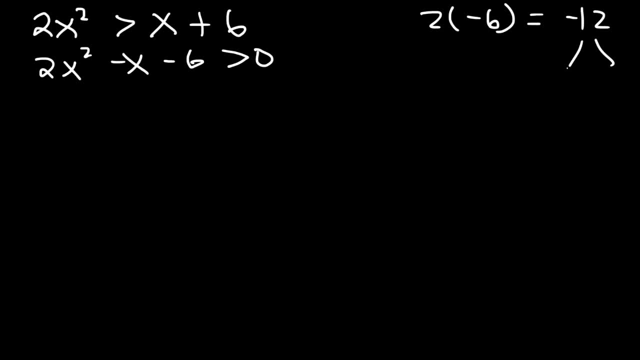 a constant term, So that will give you negative 12.. And then you need to find two numbers that multiply to negative 12, but add to negative 1, which we already know is negative 4 and positive 3.. Now what we're going to do is replace the middle term negative X with negative 4X plus. 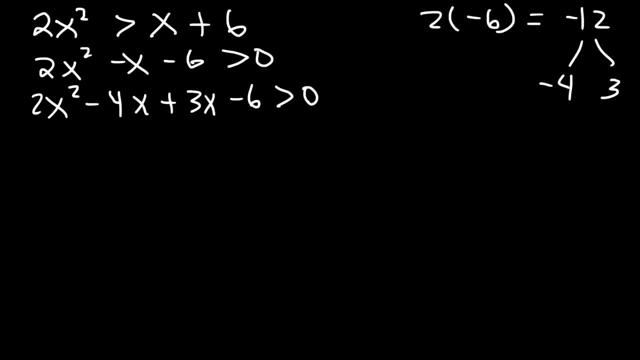 3X. So notice that negative 4X plus 3X is still negative X. So the value of the left side of the equality remains the same. Now let's factor by grouping. So in the first two terms, take out: 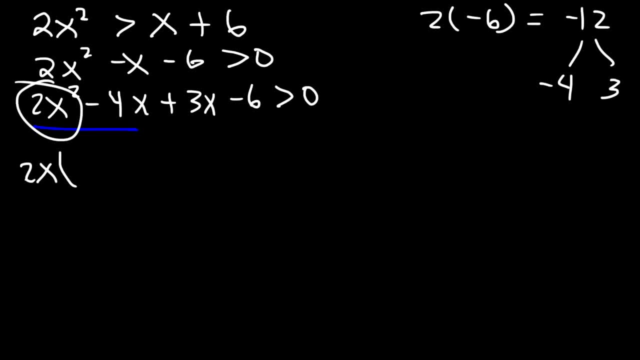 the GCF, which is 2X. 2X squared divided by 2X is X, And then negative. 4X divided by 2X is negative 2.. Now, in the last two terms, take out the greatest common factor, which is 3.. 3X divided. 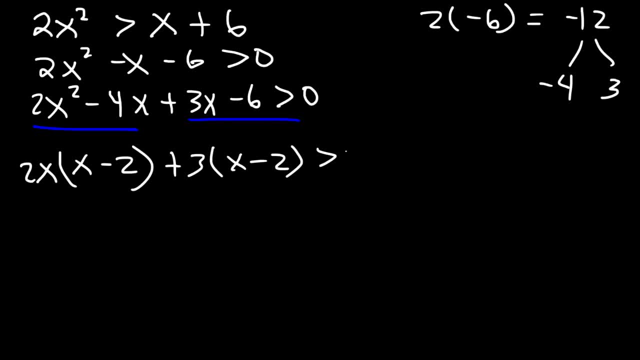 by 3 is X Negative. 6 divided by 3 is 2.. And then at this point also factor the GCF, which is X minus 2.. So if we take out X minus 2 from the first term, what we're going to have left over is 2X. And if we take out X minus 2 from 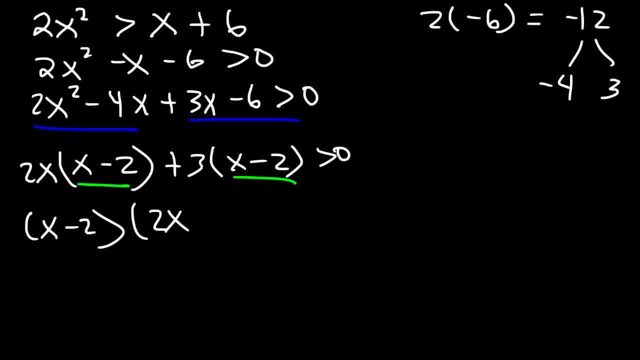 the second term, we're going to have a 3 left over, But that's going to be plus 3.. And so that's how we can factor this expression. So let's make a number line, And if we set 2X plus 3,, 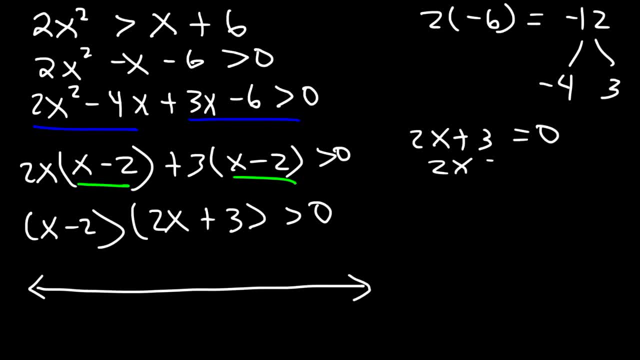 equal to 0. And if we subtract by 3, and then divide by 2,, the first point of interest is going to be negative: 3 over 2.. And if we set X minus 2, equal to 0,, the second point of interest. 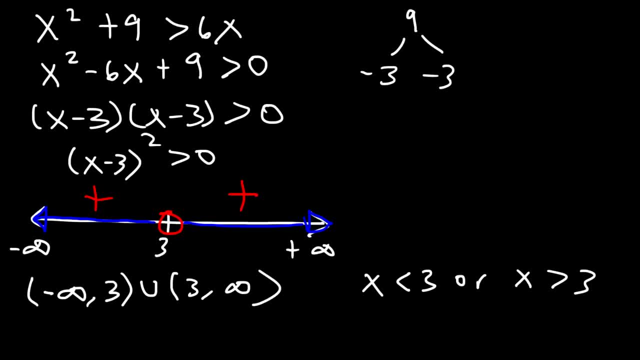 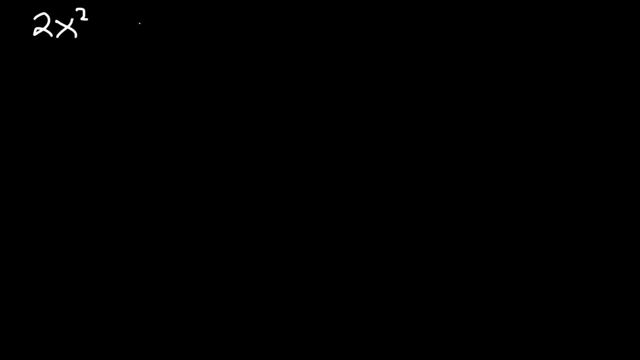 X is greater than 3, But it doesn't equal 3. So that's the solution for this particular Quadratic inequality. Now Let's move on to our next example. So let's say that 2x squared Is greater than x plus 6. Go ahead and try that. 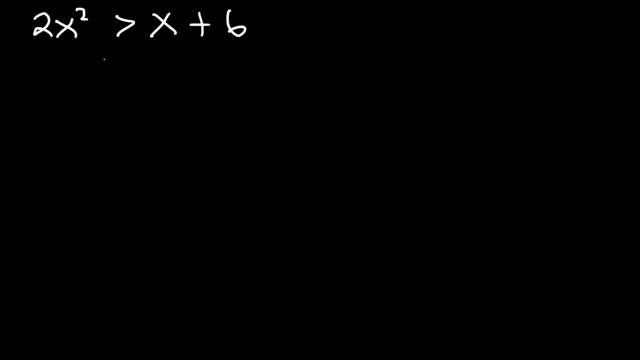 So let's move the x plus 6 From the right side to the left side. So on the left side It will be negative. Now we need to factor this expression. So how can we factor a trinomial Where the leading coefficient is not 1? First you need to multiply. 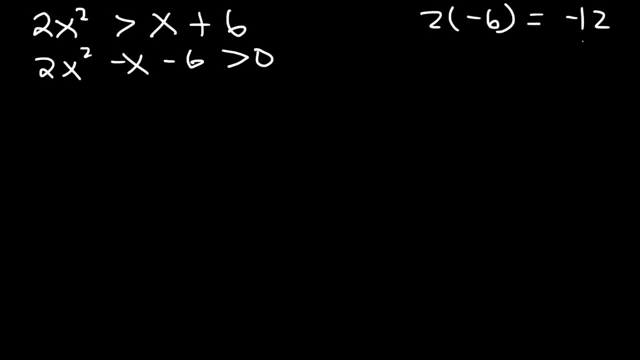 The leading coefficient and a constant term. So that will give you negative 12, And then you need to find 2 numbers That multiply to negative 12 But add to negative 1, Which we already know is Negative- 4 and positive 3. Now what we're going to do is 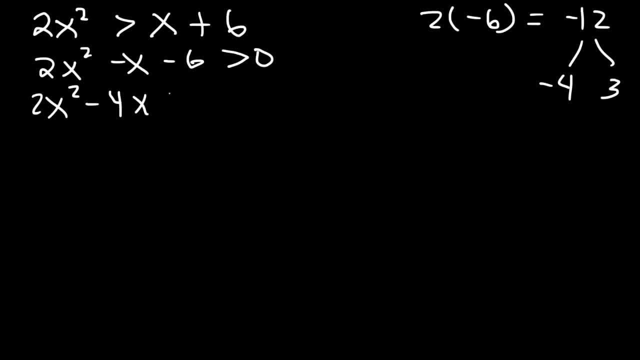 Replace the middle term negative x With negative 4x plus 3x. So notice that negative 4x plus 3x is less than 3 And negative 4x plus 3x is still negative x. So the value of the left side of the inequality. 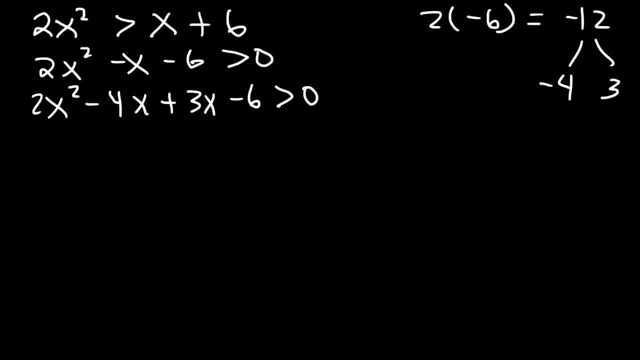 Remains the same. Now let's factor by grouping. So in the first two terms, Take out the GCF, Which is 2x. 2x squared divided by 2x Is x, And then negative: 4x divided by 2x Is negative 2. 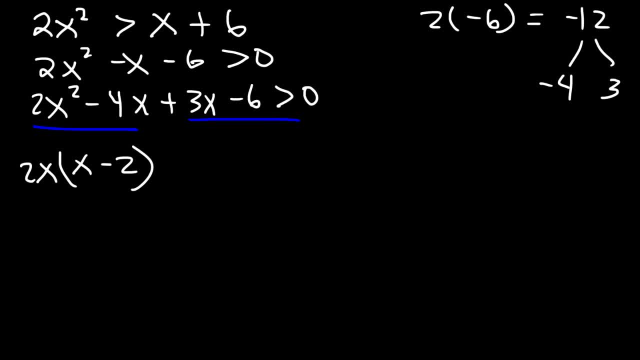 Now, in the last two terms, Take out the greatest common factor, Which is 3: 3x divided by 3 Is x. Negative 6 divided by 3 Is 2, And then, at this point, Also factor the GCF, Which is x minus 2. 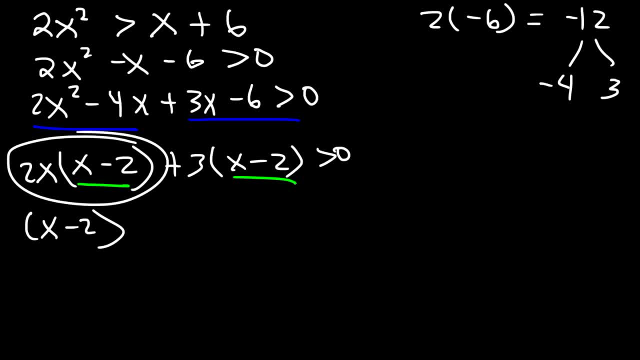 So if we take out x minus 2 From the first term, What we're going to have left over Is 2x, And if we take out x minus 2 From the second term, We're going to have a 3 left over, But that's going to be plus 3. 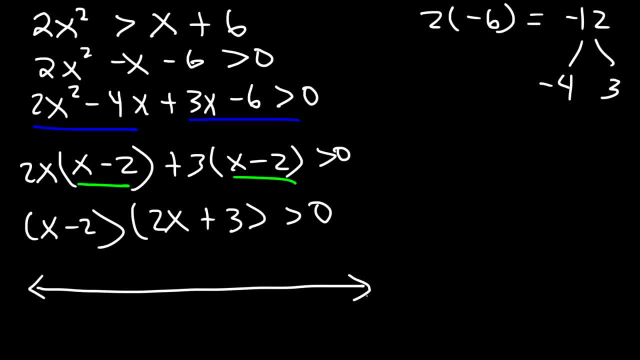 And so that's how we can factor This expression. So let's make a number line, And if we set 2x plus 3 Equal to 0, And if we subtract by 3 And then divide by 2, The first point of interest Is going to be negative: 3 over 2. 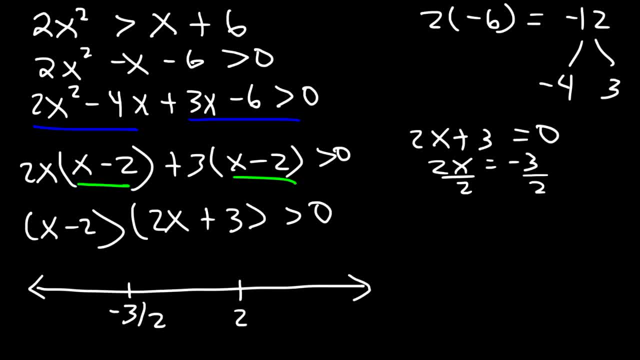 And if we set x minus 2 Equal to 0, The second point of interest Will be 2. Now keep in mind that The inequality doesn't It doesn't have an equal sign, It's just greater than 0, So we're going to take out x minus 2. 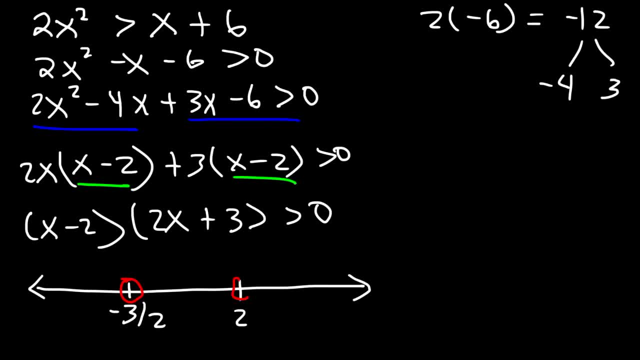 And so, therefore, We're going to have an open circle At these two points, And let's not forget Infinity and negative infinity. Now, which region do we need to shade First? let me get rid of this stuff, So let's plug in a number That's greater than 2. 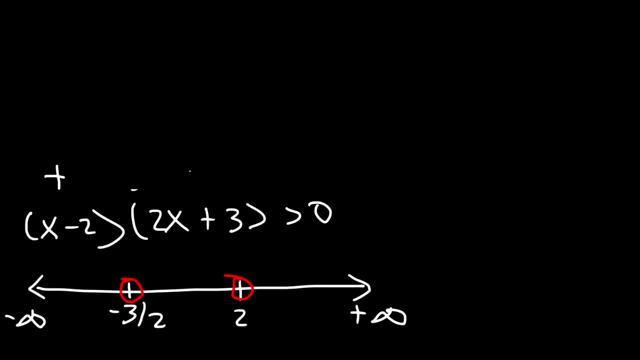 So let's try: 3, 3 minus 2 is positive. 2 times 3, Which is 6 plus 3, That's positive as well. So the right side is going to be positive. Now the multiplicity of each 0 is 1, So the signs will change. 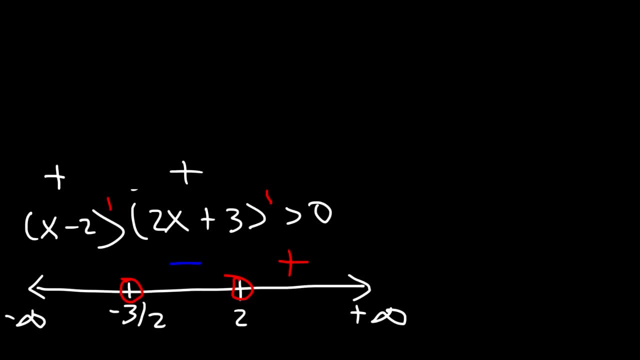 So here it's going to be negative And then it's going to be positive again. Now we want the parts where it's greater than 0, So when it's positive, That's in this region And in this region. So therefore, the answer in this region Is going to be 0. 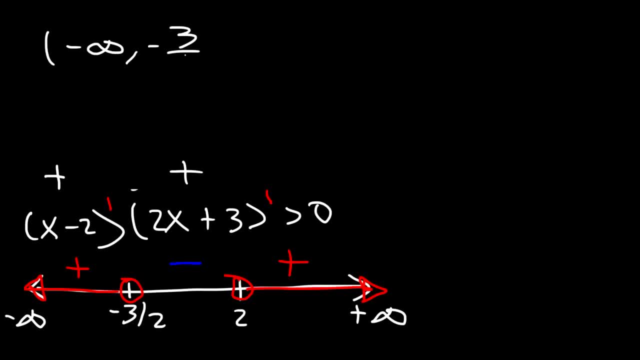 And then the final notation Is going to be: negative infinity To negative, 3 over 2, Not including negative, 3 over 2, Union 2 to infinity. So as an inequality We can say that x is less than negative, 3 over 2, Or x is greater than 2. 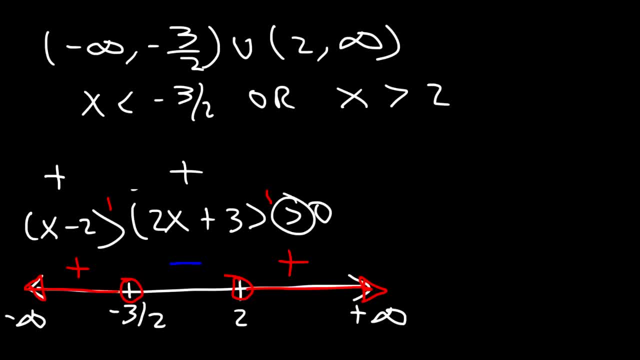 And that's it. Now let's say, for example, If it was less than 0 Instead of greater than 0. In that case we would have this region. So therefore, the answer would be, in interval notation, negative 3 over 2 to 2.. 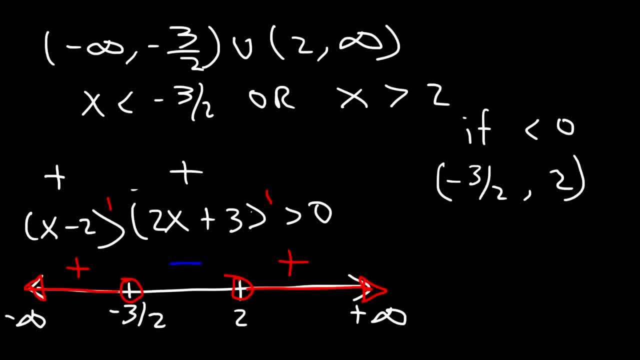 If- let me just write if- it's less than 0.. As an inequality, we could say that x is less than 2, but greater than negative 3 over 2.. Just in case you were wondering how to write it if we only had this region. 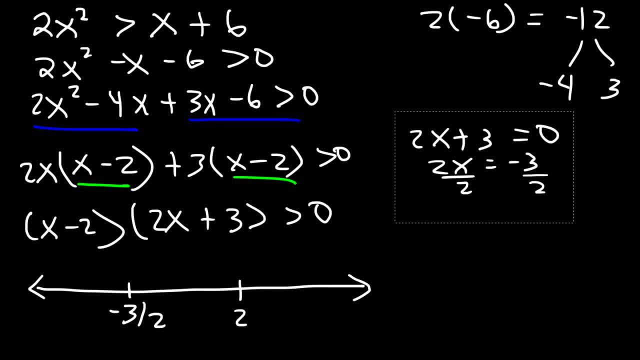 will be 2.. Now keep in mind that the inequality doesn't have an equal sign, It's just greater than 0. So, therefore, we're going to have an open circle at these two points, And let's now get infinity and negative infinity. Now, which region do we need to shade? First, let me get rid. 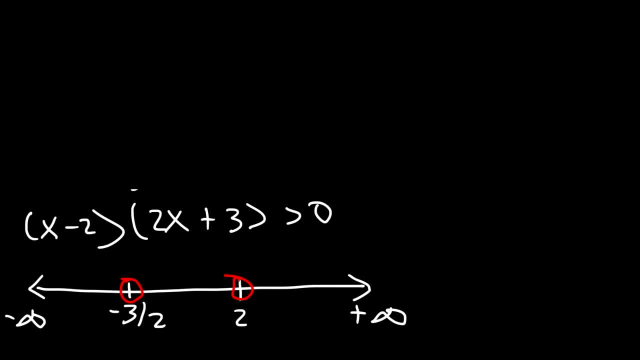 of this stuff. So let's plug in a number that's greater than 2.. So let's try 3.. 3 minus 2 is positive. 2 times 3,, which is 6 plus 3, that's positive as well. So the right side. 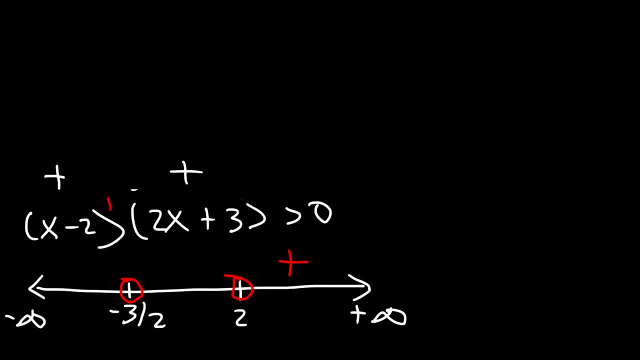 that is going to be positive. Now the multiplicity of each 0 is 1, so the signs will change. So here it's going to be negative, And then it's going to be positive again. Now we want. 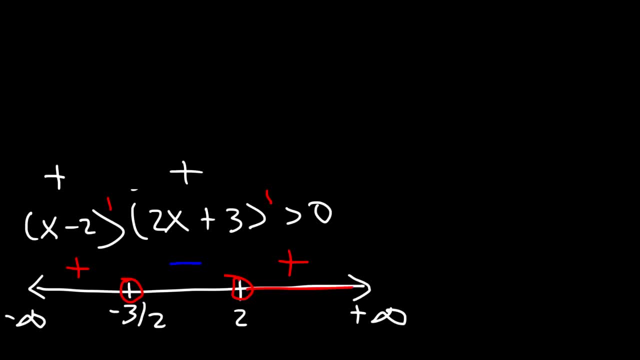 the parts where it's greater than 0. So when it's positive, That's in this region and in this region. So therefore the answer in interval notation is going to be negative infinity to negative 3 over 2, not including negative 3 over 2.. 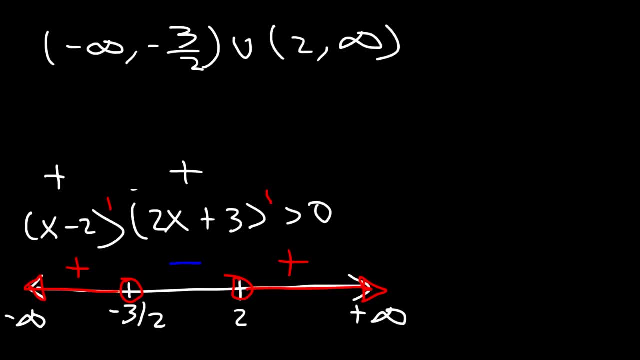 So if x is 2 minus 2, we get 0. So let's say that we want to go with this. We can say that x is 2 minus 2.. So let's say that we want to go with this, And here we want to say that x is 2 minus. 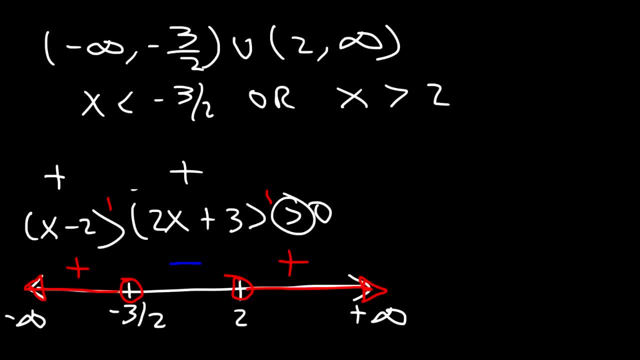 3, or x is greater than 2. And that's it. Now let's say, for example, if it was less than 0, instead of greater than 0. In that case, we would have this region. So therefore. 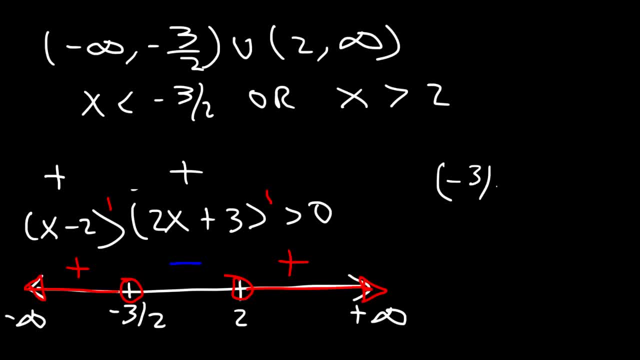 the answer would be, in interval notation, negative 3 over 2 to 2.. If- let me just write if- it's less than 0. As an inequality, we could say that x is less than 2, but greater than negative 3 over 2.. 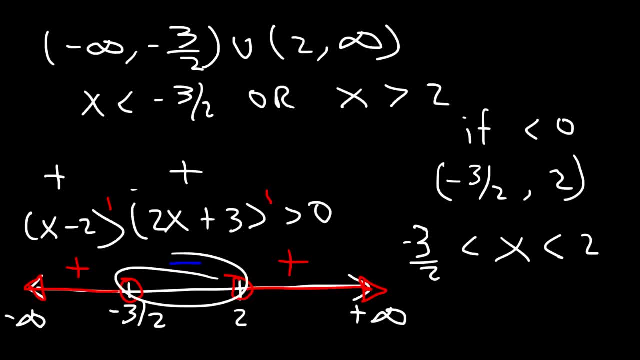 Just in case you were wondering how to write it: if we only had this region, But for this particular problem, this is the answer. So just keep that in mind. And that's it for this video. So now you know how to solve quadratic inequalities. 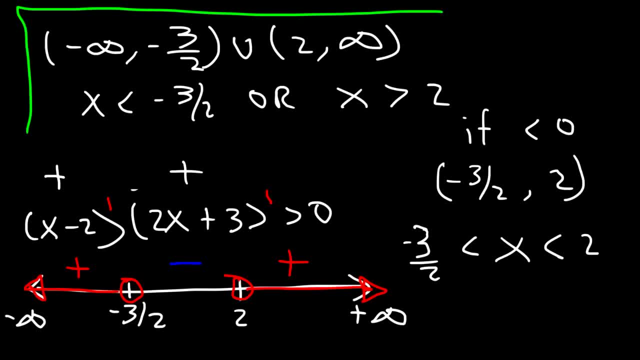 But for this particular problem this is the answer. So just keep that in mind. And that's it for this video. So now you know how to solve quadratic inequalities, And thanks for watching.